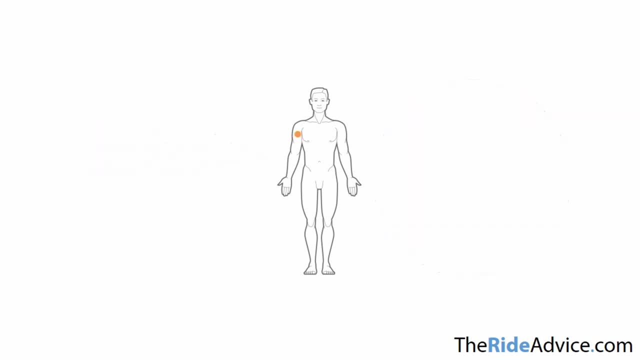 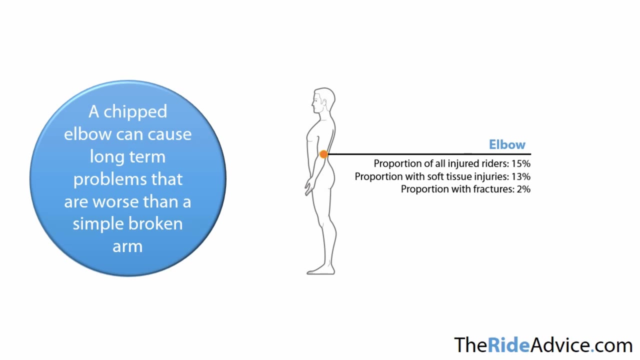 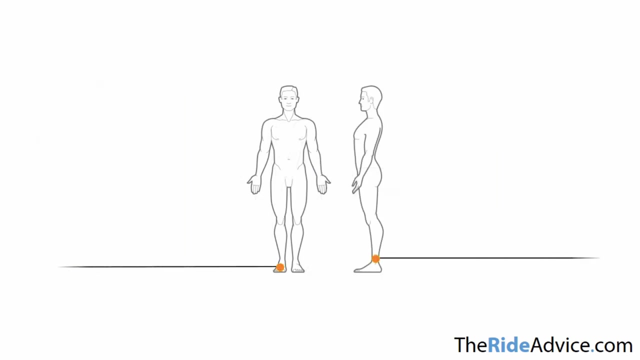 armour covering both the shoulder, elbow and your forearm. Aim for CE2 rated armour. It absorbs at least 71% more energy than CE1 armour. Be very cautious of cheaper jackets that only cover the elbow and not the forearm. Your feet are the most likely part of your body to hit the 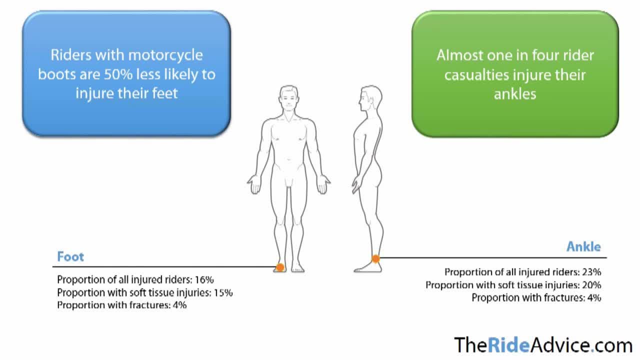 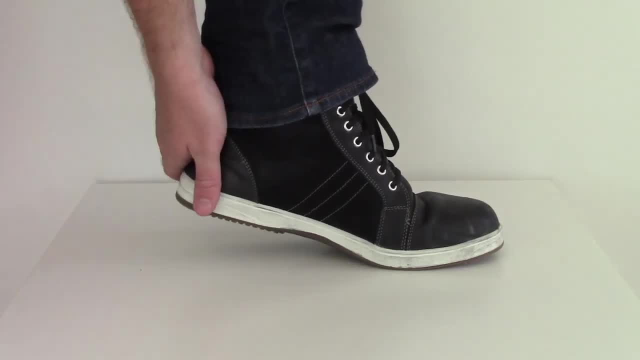 road in a crash, even more so than your hands. If you can't afford actual motorcycle boots, at least wear something like a work boot. Studies have shown they reduce the possibility of injury almost as much as armoured motorcycle boots on the street. and if you can do this with your shoes, 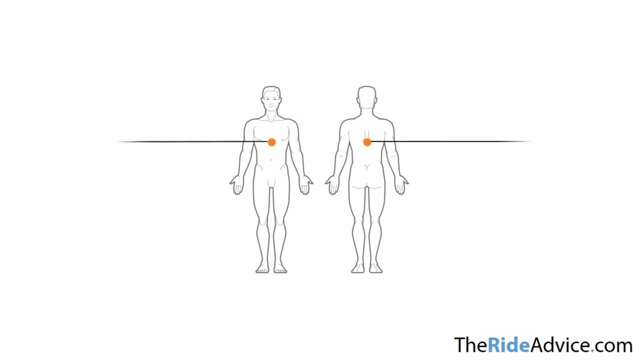 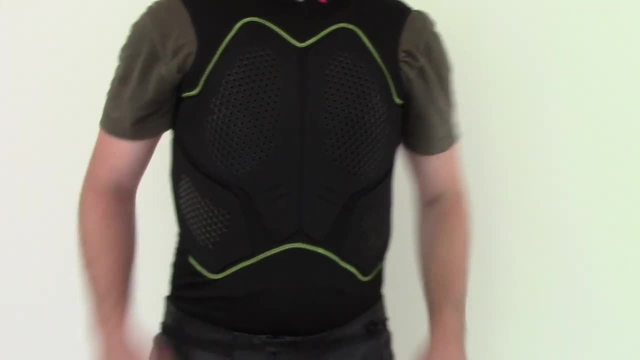 they will come off in a crash. There's little you can do to prevent spinal damage, as it's more likely that such an injury is caused by bending and torsional forces on the spine, and not direct impacts that a back protector is designed for. They will at least, however. 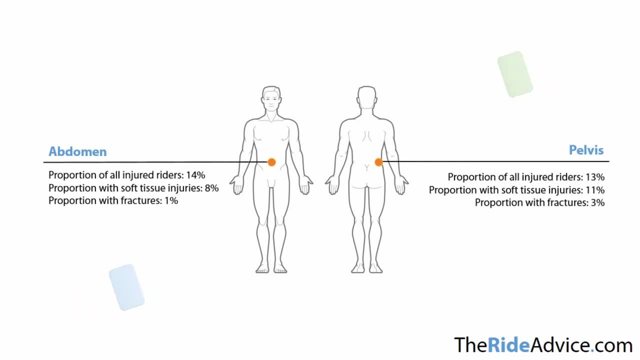 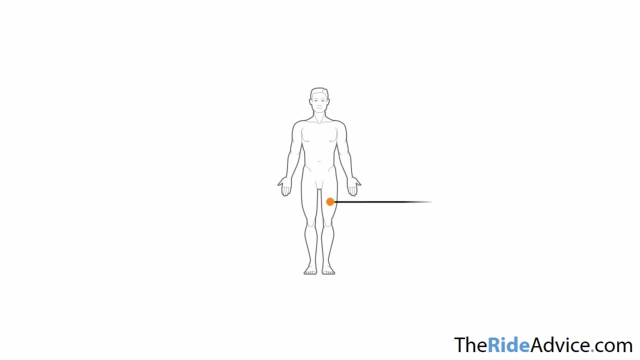 reduce bruising and tissue damage from a slide. Padding on your hips can assist here, as it will absorb some of the energy, reducing those torsional forces. Keep in mind that most Kevlar jeans don't come with knee armour and almost none offer protection on the hip or thighs. This means 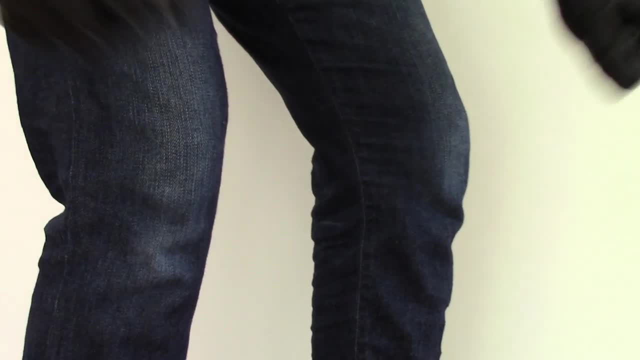 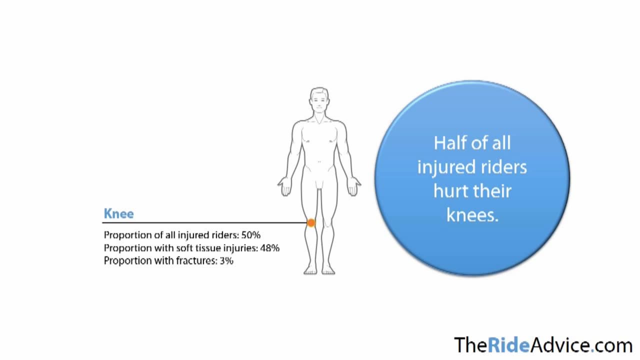 that while they reduce abrasion injuries, they won't do anything to minimise bruises or fractures. Most textile pants and Kevlar jeans that don't come with armour at least have the provision for you to add it in later. There really isn't a huge amount you can do to prevent a fracture. 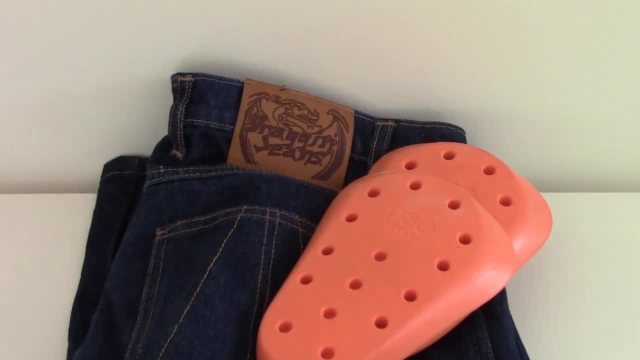 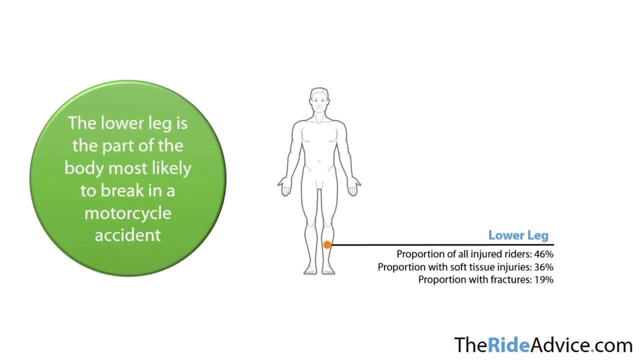 to your legs in a serious enough crash. The forces exerted on a body spiralling in the air or hitting another object mean the current armour can only do so much, But they will greatly reduce cuts, bruises and sprains. High boots with some shin protection, which 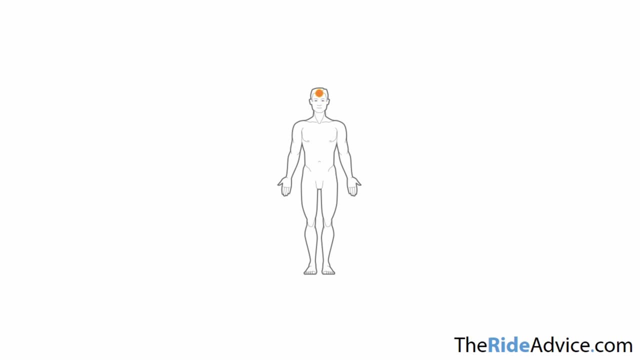 overlap the armour in your pants will also help. In one study, over 80% of riders with head injuries were either not wearing a helmet or it came off. Type of helmet is important, with riders who choose to wear an open face helmet 25% more likely to sustain an injury. 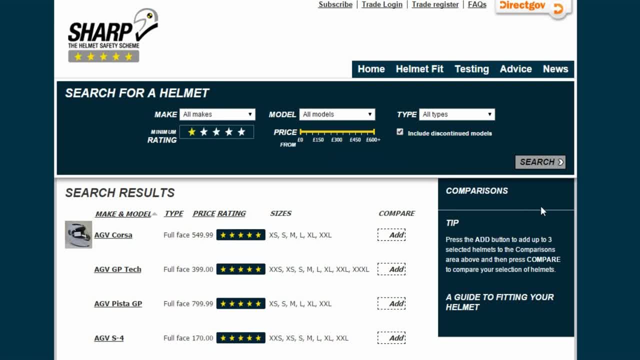 than those that wear full face helmets. And to ensure the helmet you're buying is safe, visit the UK government's website, SHARP, which does crash testing on various motorcycle helmets.